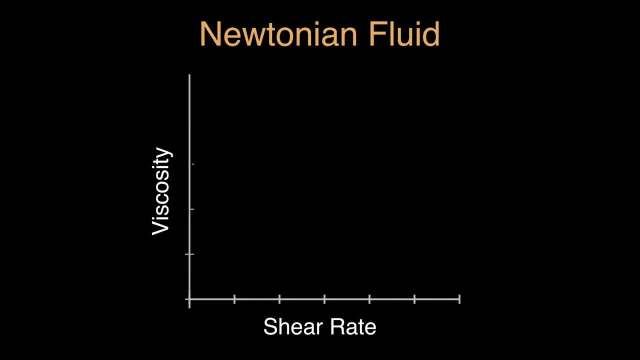 summarize it for you: When we call a fluid Newtonian, it means that the rate at which we apply some shear stress has no effect on its viscosity. An example from this answer on StackExchange is ketchup. When we have difficulty removing ketchup from a bottle, we hit the bottom of the bottle. 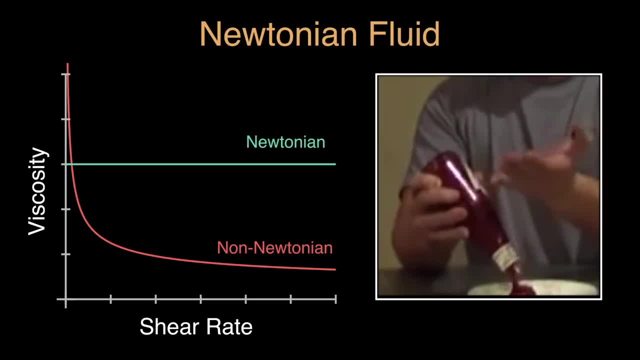 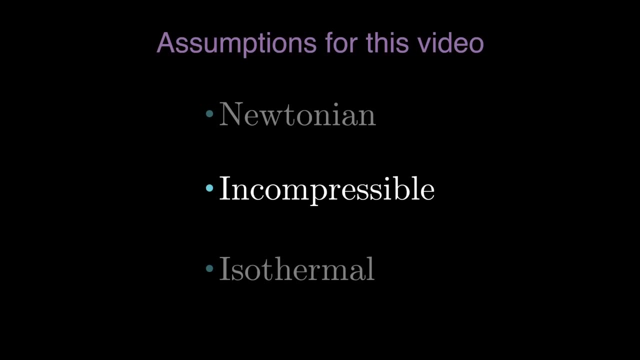 and the ketchup comes out with ease. Looking at ketchup's shear rate vs viscosity graph, we can see that hitting the bottle, which increases the shear rate, decreases its viscosity, which lets the fluid out. The second assumption is that the fluid is incompressible. It means exactly what you. 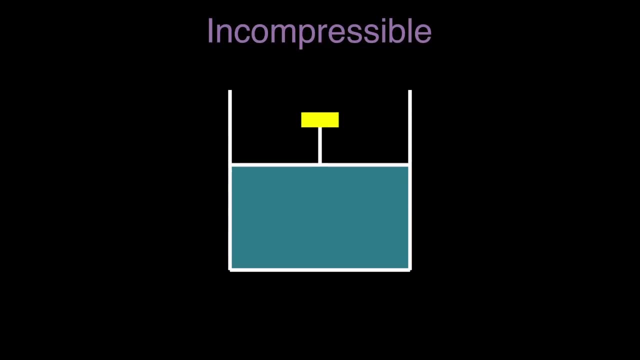 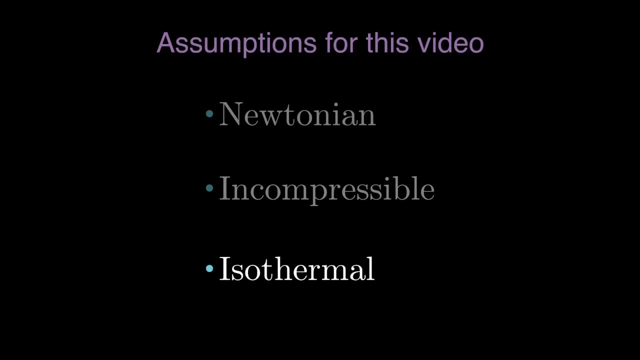 think If I compress the fluid that is at pressure, there's no considerable variation in of the fluid. The last assumption is that the fluid is isothermal. This just means that as the fluid flows, there's no loss or gain of heat. And this takes us to the Navier-Stokes equations. 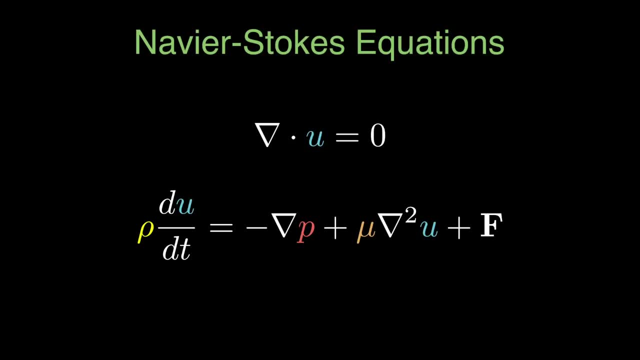 As daunting as they may seem, they're actually based on quite well-known physics properties. Note that when we talk about fluids, we typically talk about an infinitesimal volume of fluid, and so we're trying to describe the motion of each individual molecule rather than the fluid as a 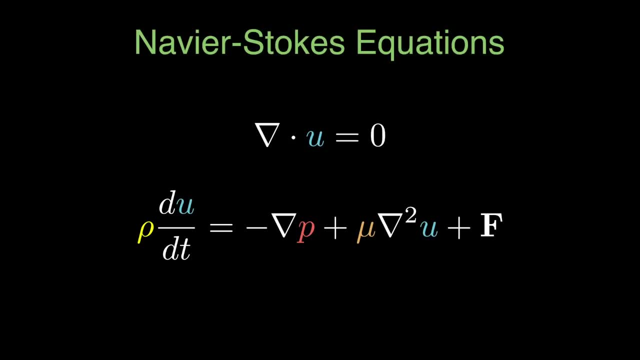 whole. This first equation right here tells us that mass is conserved within the fluid. The operator here is called the divergence of a vector field. The vector field in this case u is the velocity vector field of the fluid. A vector field is what you get when you assign every single point in space to a vector. 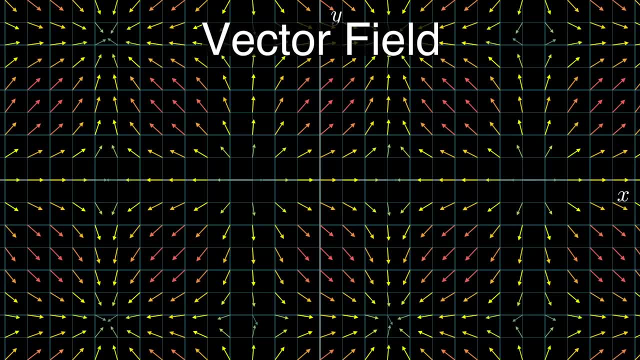 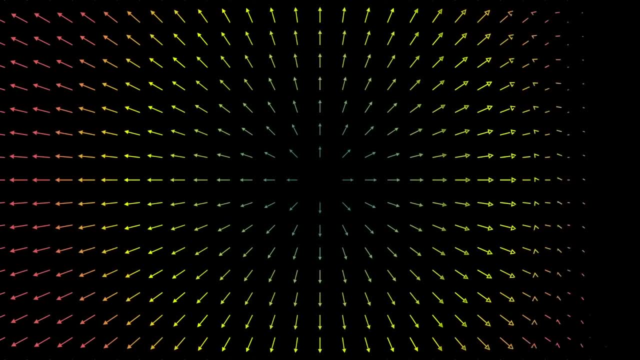 Vector fields can describe many things, from fluids to electric fields, to gravitational fields and so on. The divergence of a vector field is an operator that tells us how much a point tends to divert vectors away from it. Consider this vector field. It appears that vectors seem to be moving away from the origin. 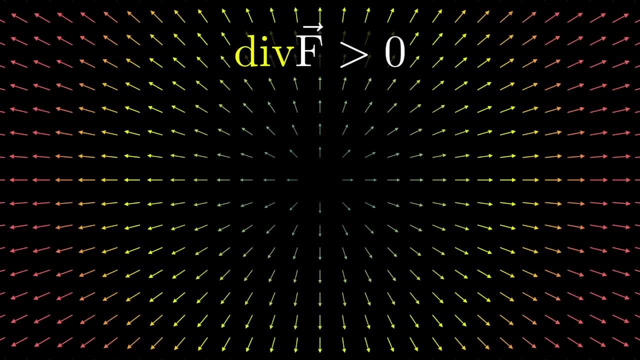 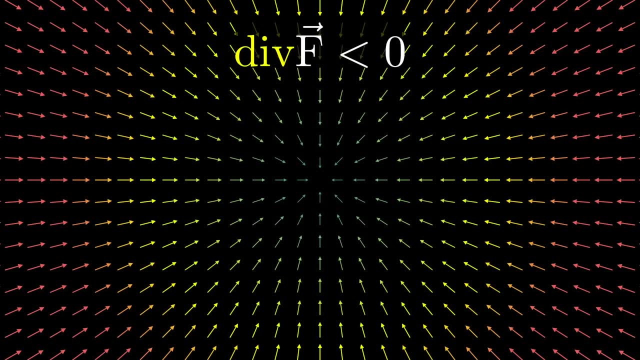 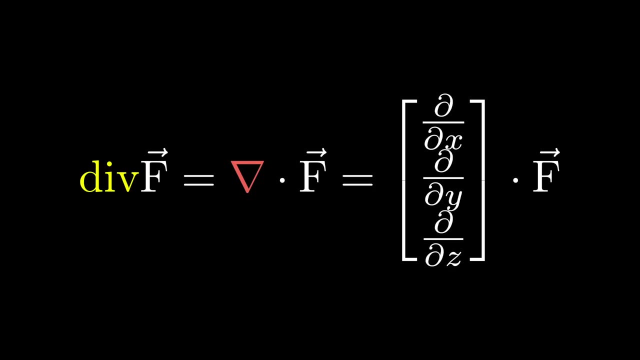 This indicates positive divergence. Similarly, this vector field seems to have vectors that flow into the origin. This indicates negative divergence. Numerically, we write the divergence as a dot product between the gradient vector and its vector field. This fantastic video by 3V1Bar. 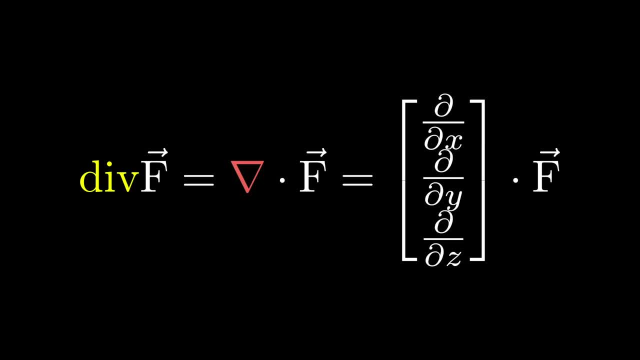 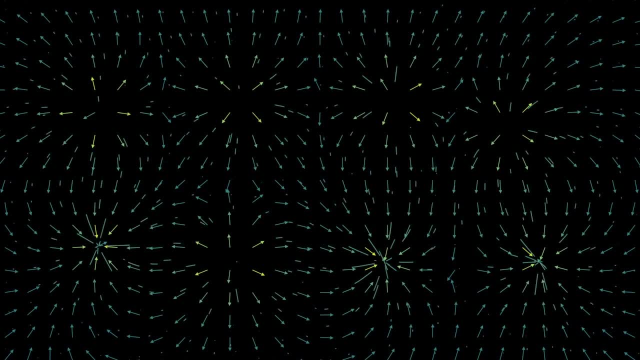 explains why. if you're interested, check it out. In terms of fluids, the divergence of a vector field indicates how much or how little a point acts as a source of a fluid. If we imagine water in some area, it's impossible for the water to. 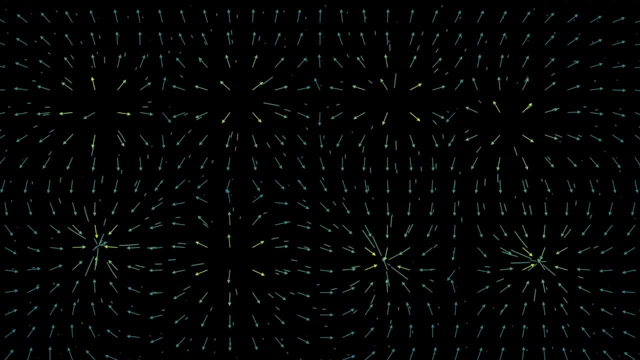 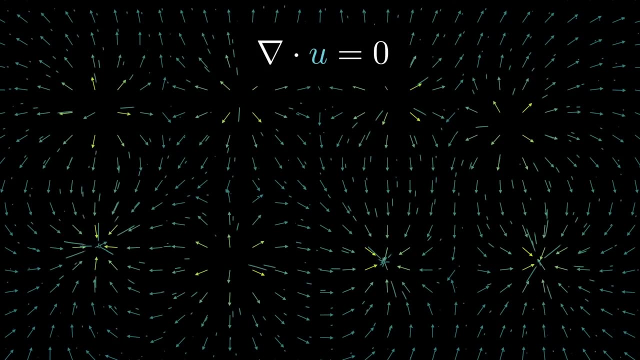 simply disappear. It could either change forms when mass is never destroyed, and thus the divergence across the fluid has to be zero, and hence the first Navier-Stokes equation. This second equation is just a rewritten version of this equation. It is just a rewritten version. 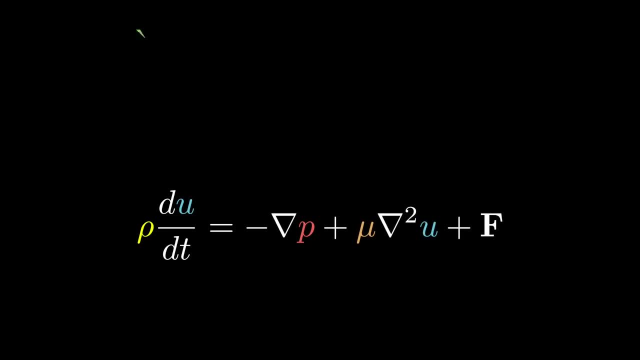 written version of Newton's second law. If you remember, Newton's second law tells us that the sum of forces acting on a body can be written as its mass times the acceleration. Considering this for a single molecule of a fluid, let's see how we can derive the. 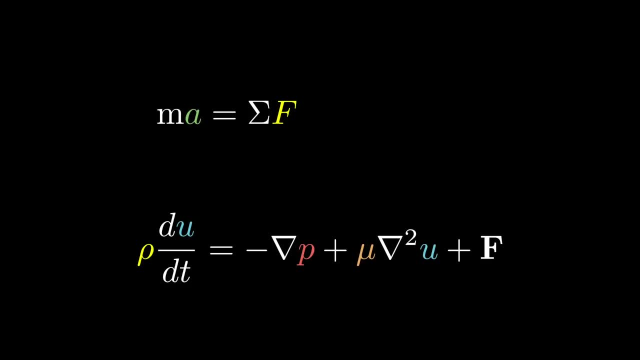 second Navier-Stokes equation. First of all, since we're considering each individual point, let's replace mass with density. The mathematical reason behind doing this is that, to consider each point, we have to divide by volume, and mass by volume is equal to density. Next, let's 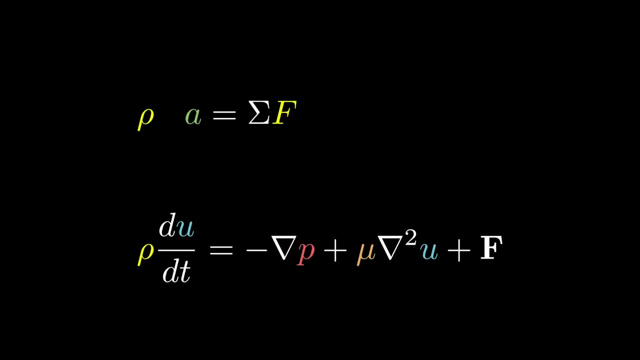 consider acceleration. Well, we have the velocity vector field U and we know that the acceleration is just the derivative of the velocity vector field. So we can replace A with du by dt. A quick side note: you might see this bar written as del U by del t plus u dot grad. 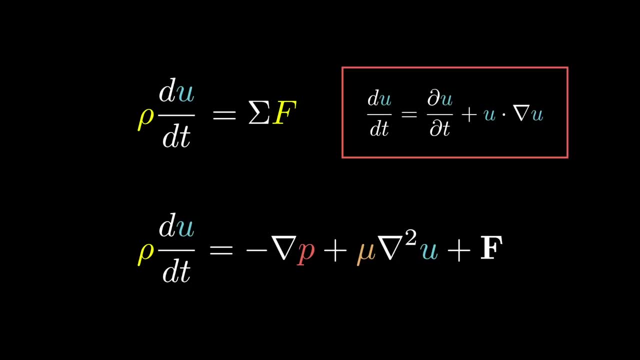 u. This is essentially the same thing. When we expand du by dt, we use the chain rule which gives us this variable where expression? Now we need to consider what are all the forces acting on this molecule of a fluid. We can break this down into internal forces, which are: 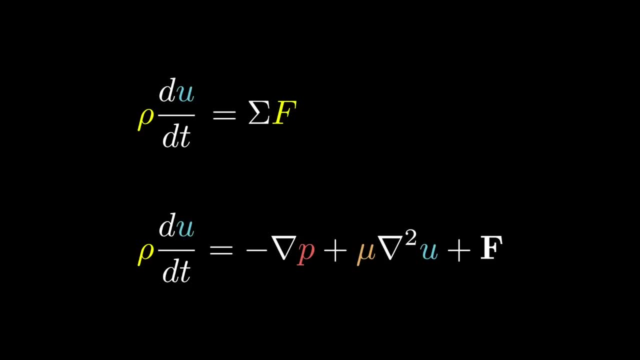 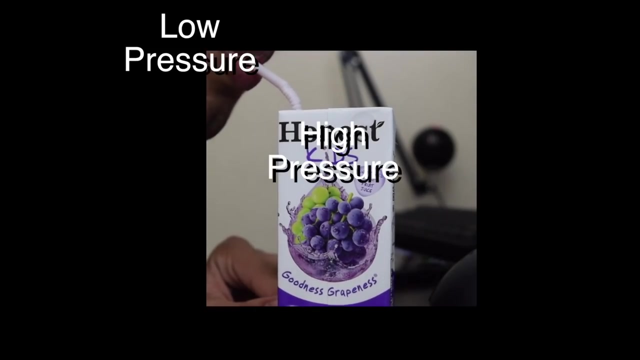 forces exerted by the molecule of the fluid itself, and external forces, which are forces exerted by some external object. The first internal force we take into account is pressure. Consider drinking from a straw. Sucking on the end of a straw creates an area of low pressure which forces the drink to move. 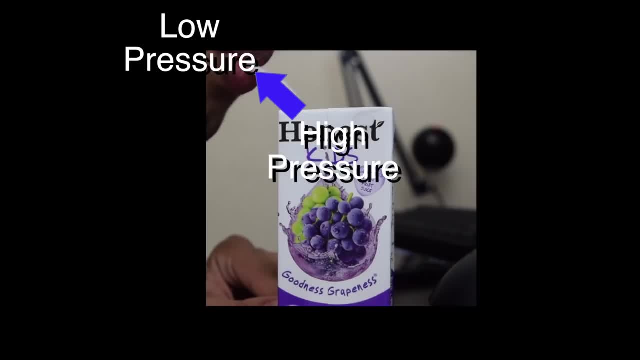 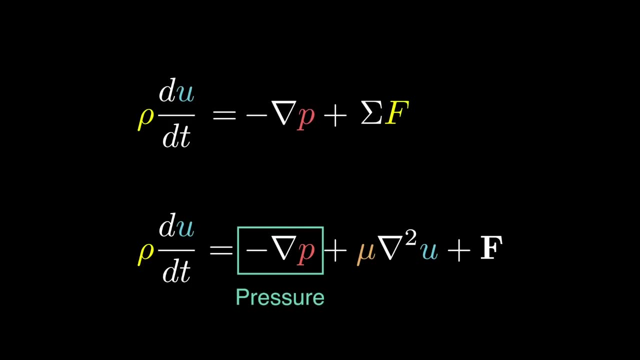 from the area of high pressure, which is below, to the area of lower pressure. This force is dependent on the change in pressure, or the pressure gradient, which we can write as grad of P. The second force we factor in is friction, or viscosity. If I pour water into a cup, the water moves quite fast, whereas if I'm 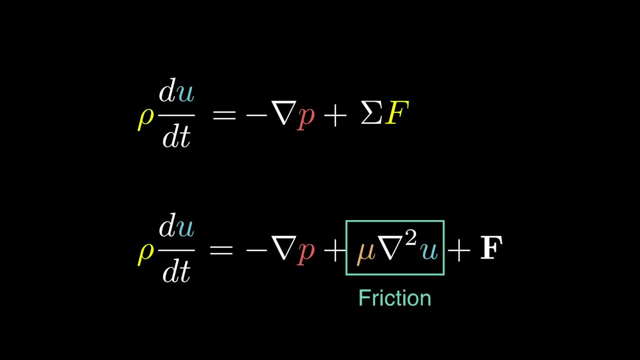 pouring honey, it moves quite slow. This is because there's a lot more friction between the molecules of honey compared to the molecules of water. The mathematical way of writing this force for Newton's law is to write the force of water as the force of water. The mathematical way of writing this force for Newton's law is to write the. 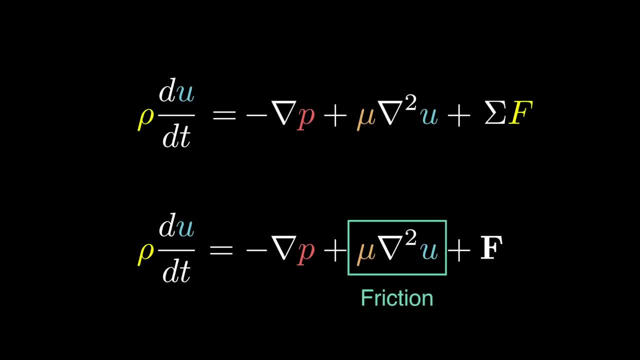 force of water as the force of water, The mathematical way of writing this force for is this expression right here. I'm not going to go into that as to how this equation arises, but I've left a few resources you can use to read up about. 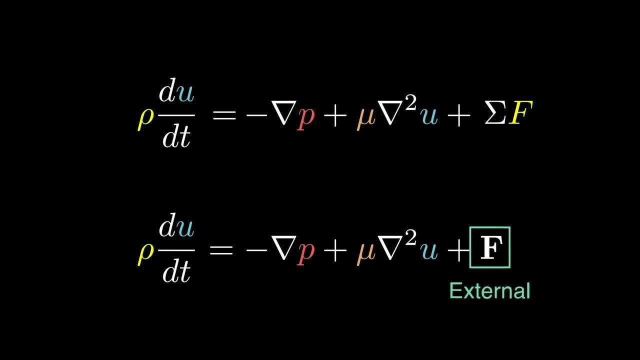 this and finally, to account for the external forces, we just denote any external force by the letter F. It's pretty common that gravity is the only external force, so we sometimes write rho times G instead of F, and this is why the Navier-Stokes equations can model any fluid. they're 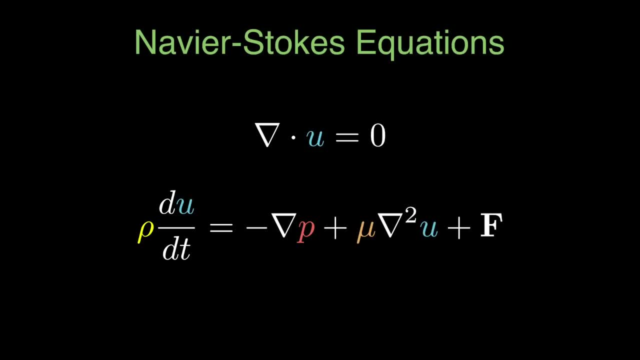 simply to fundamental controls: R times G, because they can τοdoor any fluid in another fluid. fundamental laws of physics written out for fluids. So why do these equations have a million dollar price attached to it? Well, to answer that, let's just look at the actual problem. 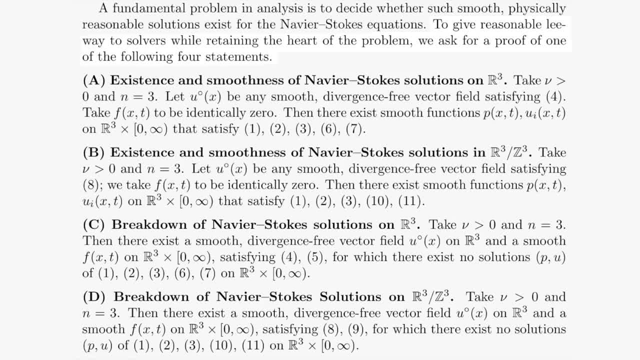 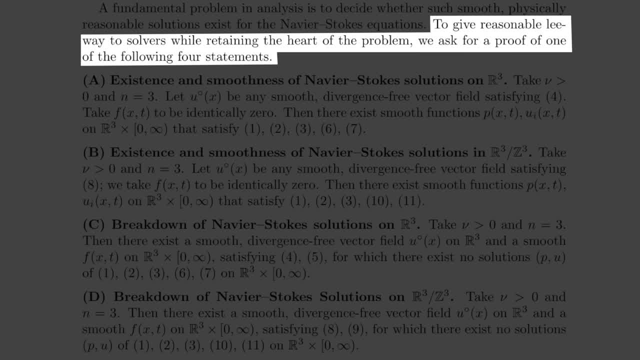 from the Clay Math Institute. It goes as follows: To give reasonable leeway to solvers while retaining the heart of the problem, we ask for a proof of one of the following four statements. The first two questions ask for a smooth solution to the Navier-Stokes equations. Let's break. 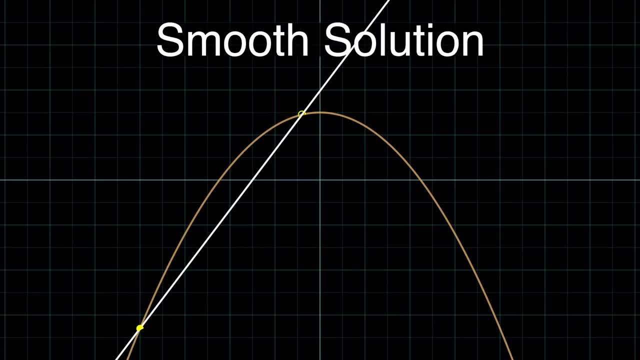 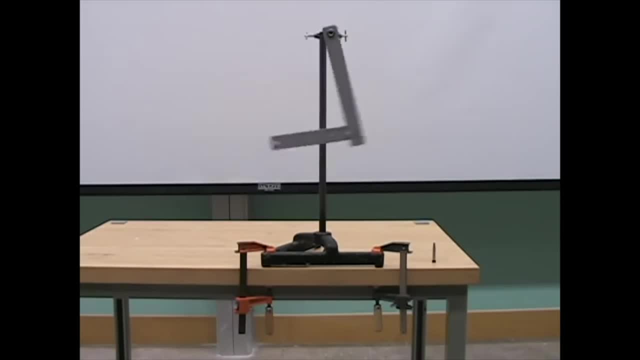 down what this means. When we say that a solution is smooth, mathematically, it means that the solution is differentiable. Chaotic doesn't mean that it's random. It simply means that if I slightly change the initial condition, it results in a large change in the outcome. 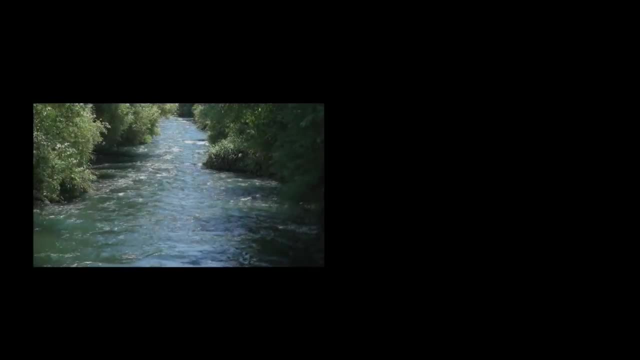 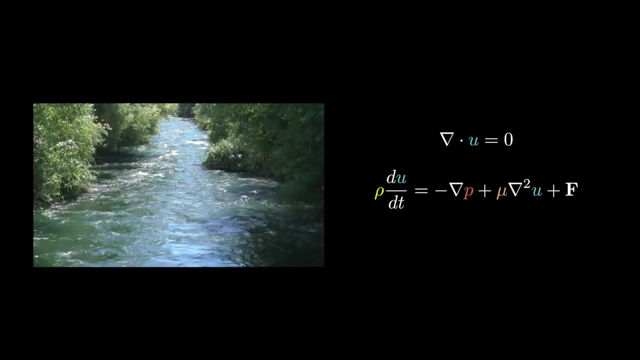 And this is where the question gets incredibly difficult. Sure the Navier-Stokes equations. lets us take some state of a fluid and let us predict what will happen in the future. but the chaotic nature of the fluids, with turbulence, makes it incredibly hard to make. 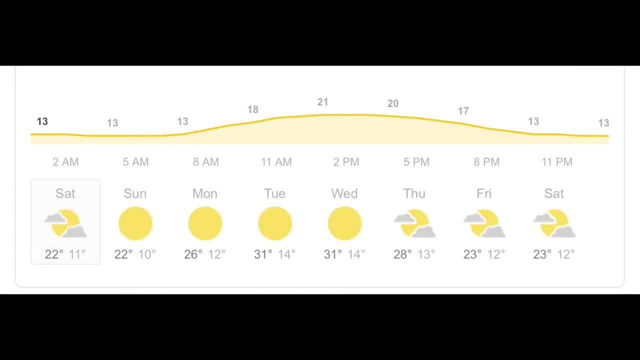 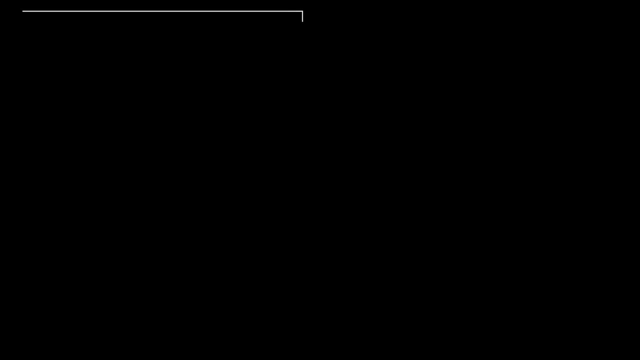 long-term predictions. This is why we can't predict the weather for more than seven days. This is also why we can't predict the weather for more than seven days. This is also why we can't predict when we're going to have turbulence on an airplane. 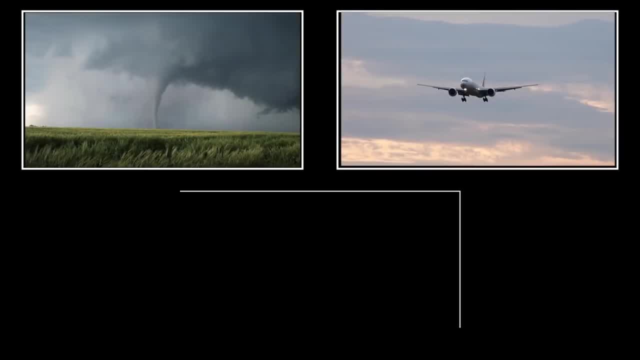 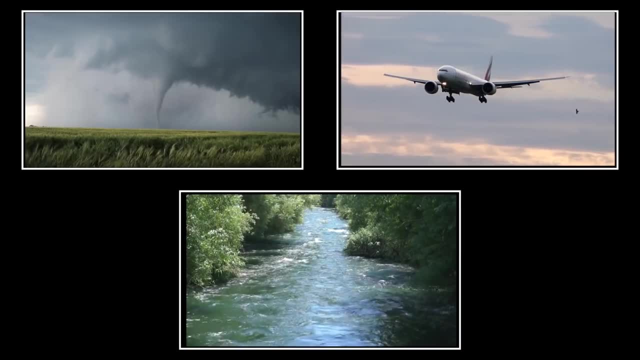 Despite this, the Navier-Stokes equations are incredibly useful. They're used extensively to model aerodynamic objects, for example a plane or a car. Like I mentioned before, the weather forecast also relies on the Navier-Stokes equations. It still remains one of the most